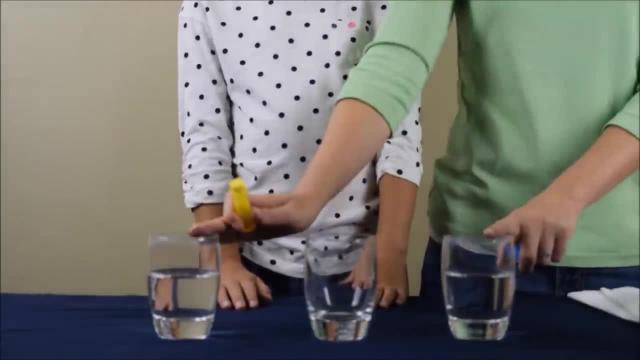 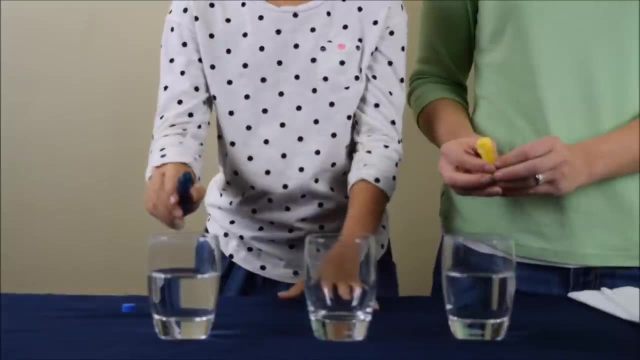 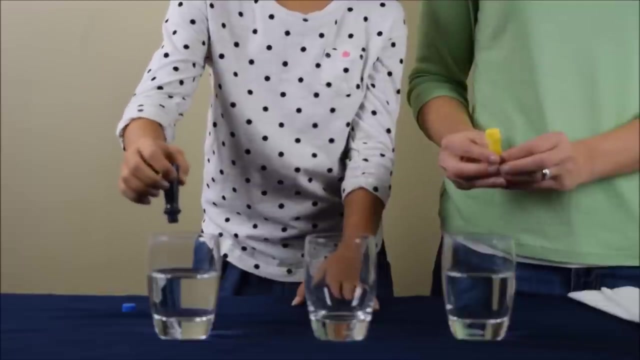 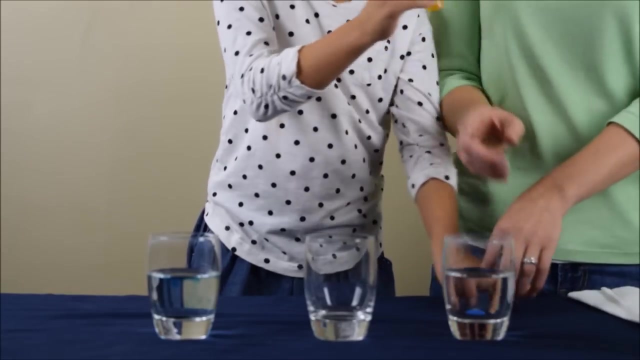 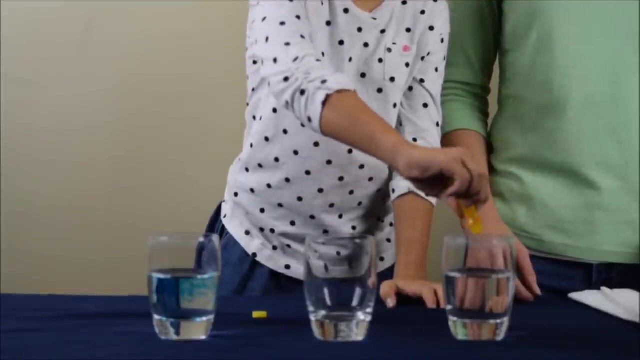 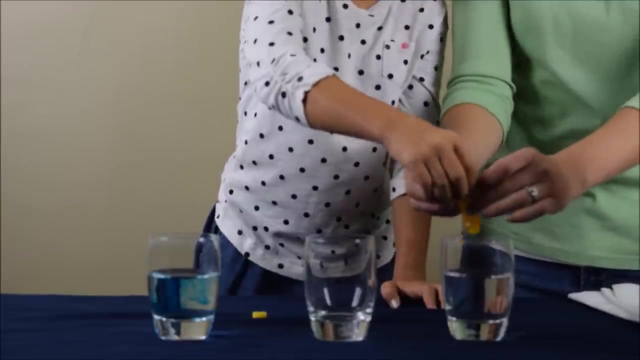 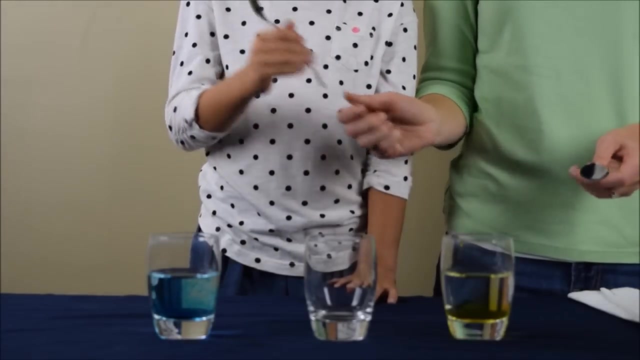 so, now that we have the water in the glasses, we're going to dye the water with some food coloring and we are going to use some blue food coloring for this glass, okay. and we're going to use some yellow food coloring for this glass, okay. so, now that we have the food coloring in, we are going to mix, mix the. 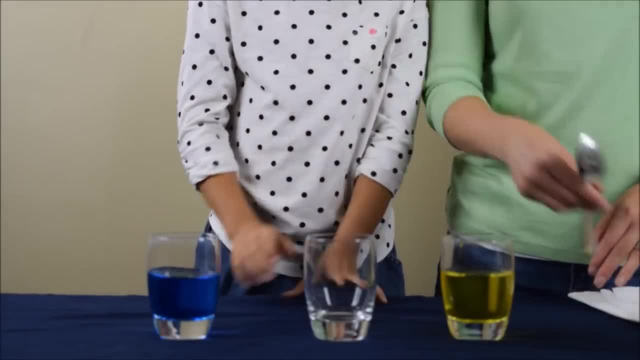 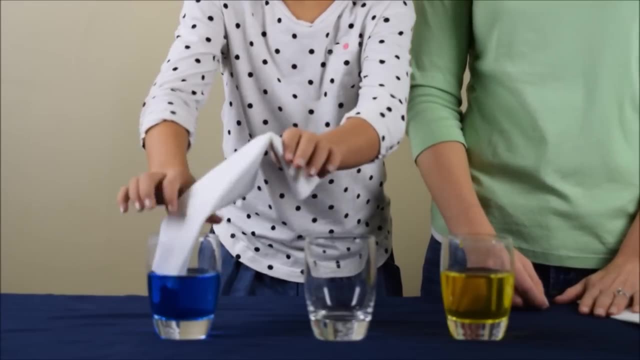 water. so the food coloring is completely blended in with the water. it's completely mixed. we're going to go back to our paper towel and again, this is our first paper towel and we're going to put one end into the blue water and then one end into the empty glass, just like that. we're going to take the second paper. 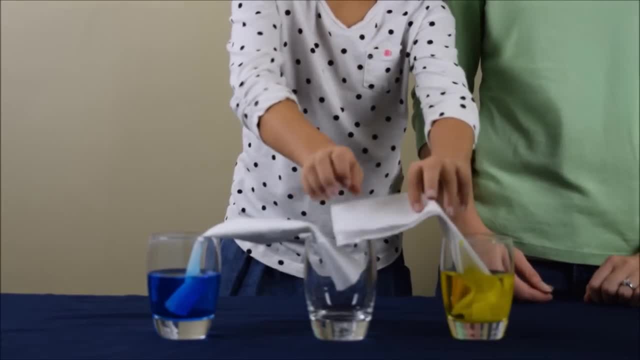 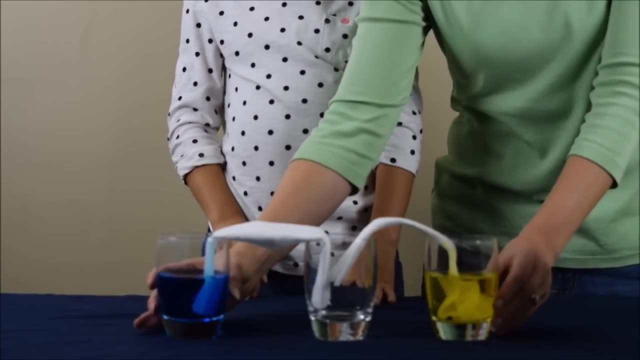 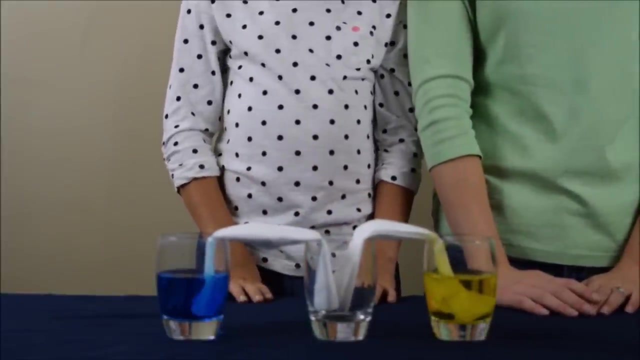 towel, and we're going to put one end into the yellow water and one end into the empty glass, and I think I'm gonna move this one just a little bit closer than that. one, too, got itso. now the paper towels are in the glasses appropriately, and it is time. 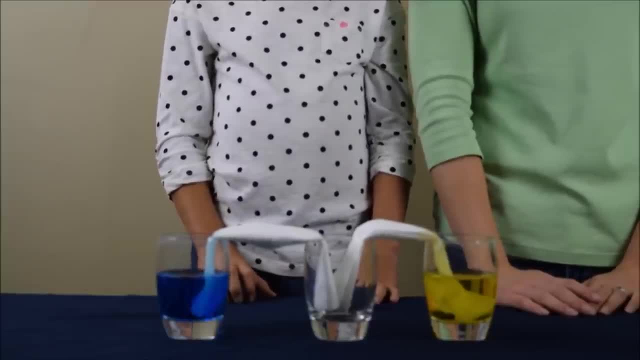 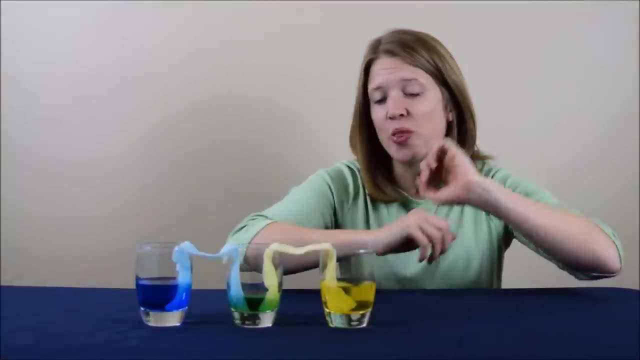 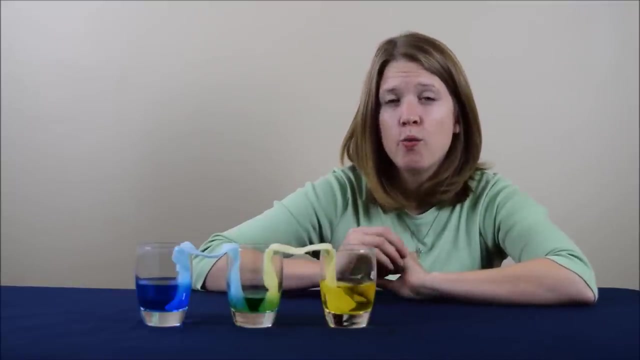 for us to wait, so we are gonna let them sit like this for about an hour, and then we're going to check back. we are back to check on the walking water science experiment, and it's been a few hours since we last checked it in. If you remember, though, when we first put the paper towel into the water, the water. 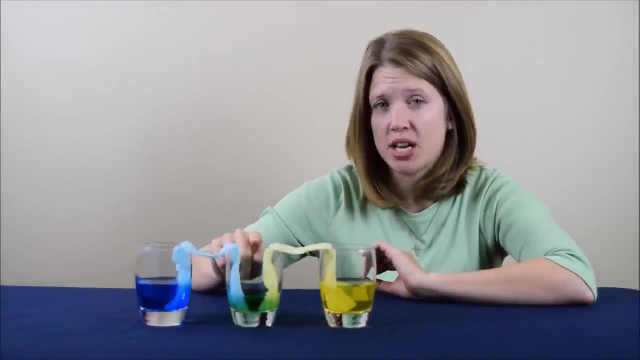 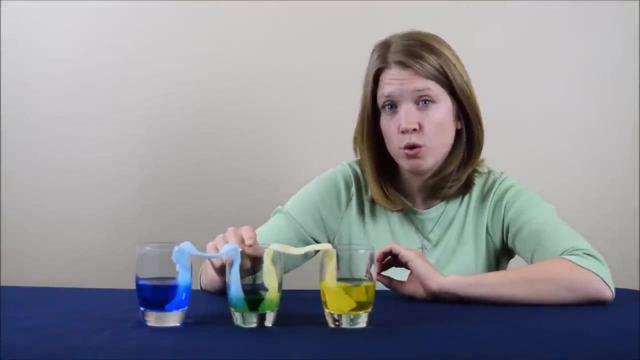 almost immediately started walking from one glass across the paper towel to the other, So you don't have to wait that long. However, the longer you wait, the fuller the glass in the middle will be. So let's take a look at the experiment. So we notice that here. 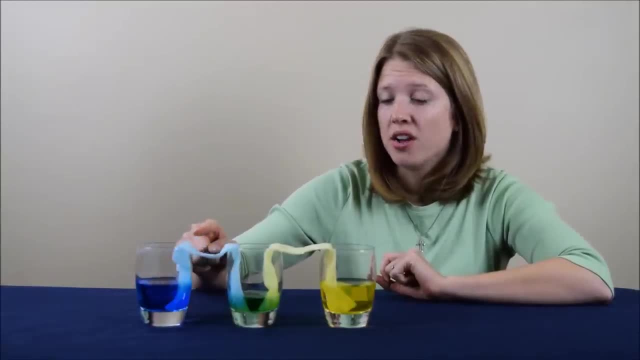 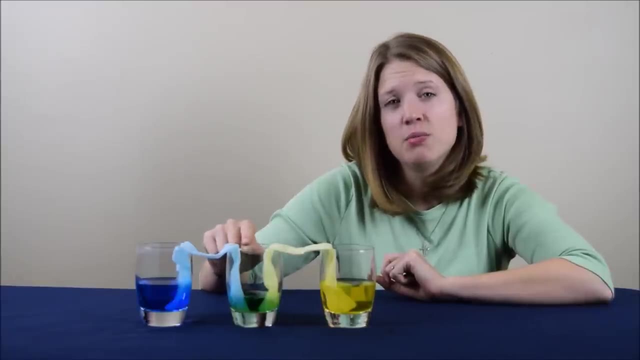 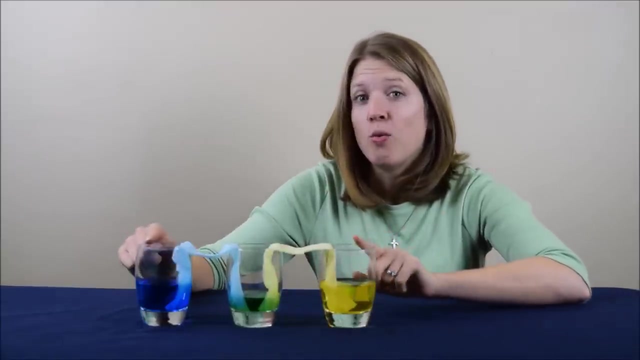 the blue water that was in this glass has walked across the paper towel into the middle, And some of the yellow water that was in this glass has walked across the paper towel and into the middle glass. So I have two questions for you. The first one: why did the water